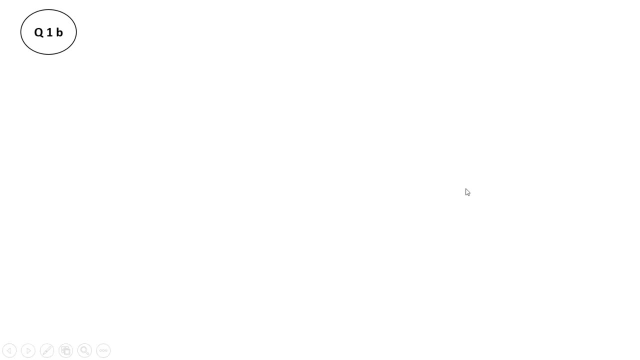 in this video we will try to understand how to solve examples on entropy in case of thermodynamics. so we have taken this example from Pune University question paper and it is question number 1 B. a copper block of mass, 1 kg at 500 Kelvin is emerged in a lake which is at 300 Kelvin till it reaches the thermal. 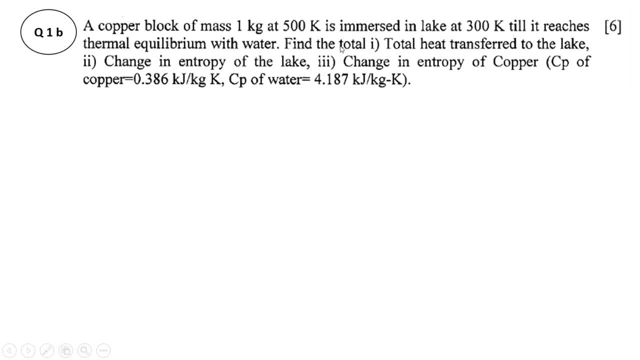 equilibrium with water, find the total heat transfer to the lake, then change in entropy of the lake and change in entropy of copper. CP of copper is given as 0.386 kilojoule per kg Kelvin and CP of water is given as 4.187. 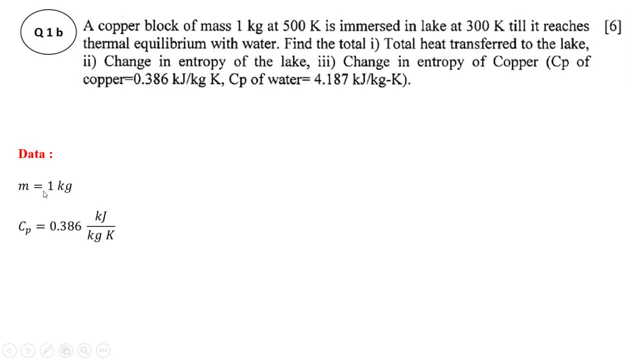 kilojoule per kg Kelvin. so mass of the block: it is given as 1 kg CP of copper. it is given as 0.386 kilojoule per kg Kelvin. then temperature T 1 of the copper block is 500 Kelvin. that of lake in which it is emerged is 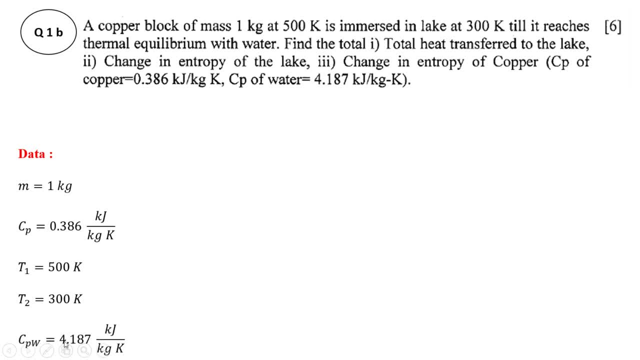 300 Kelvin and CP of water is given as 4.187 kilojoule per kg Kelvin. now the first thing that we have to find out over here is the total heat transfer to the lake. so Q is equal to integration of t1 to t2, MCP, DT or Delta T. so MCP is 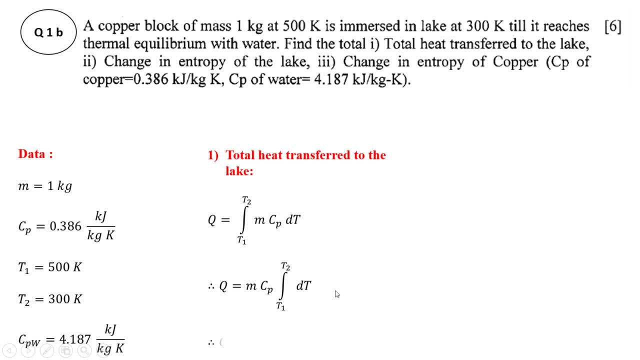 constant, so it is only integration of DT. integration of DT is T and the limits are from t1 to t2. so substitute the upper limit in place of the upper limit, that is t2, minus the lower limit, that is t1. so mass is 1, CP is 0.386 and it is. 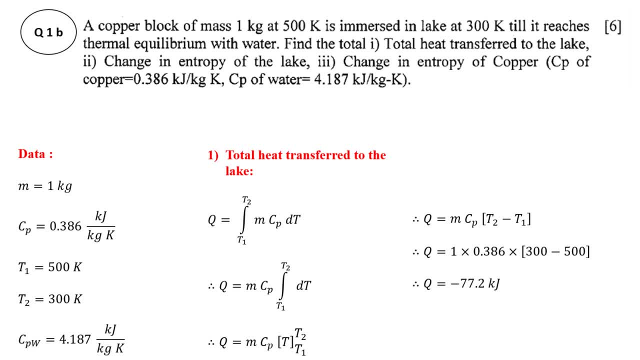 300 minus 500. so Q is equal to minus 77.2 kilojoule. so heat is transferred. that heat that is transferred to the lake is 77.2 kilojoule and the heat is transferred from the copper plate to the water, so the heat transfer is 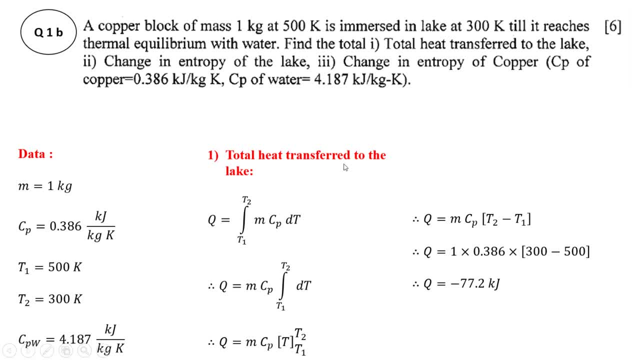 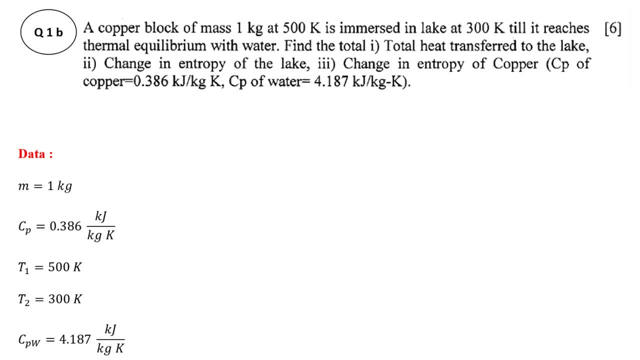 transferred to the lake, so as the copper block it is losing the heat. the negative sign is there. the second thing that we have to find out is the change in entropy of the lake. so change in entropy of the lake is equal to heat transfer to the lake divided by temperature of the lake. the lake is 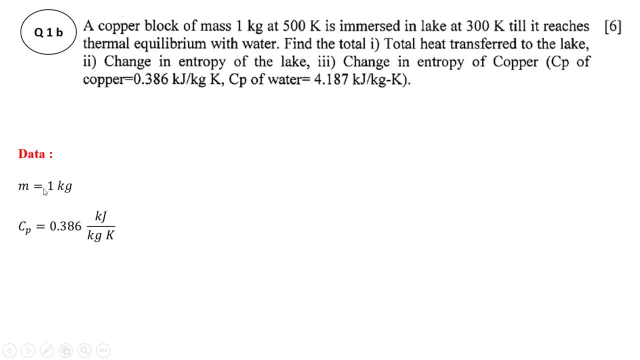 seven kilojoule per kg Kevin. so mass of the block it is given as one kg CPF copper. it is given as zero point three, eight six kilojoules per kg Kelvin. then temperature d1 of the copper block is 500 Kelvin, that of lake in which it is. 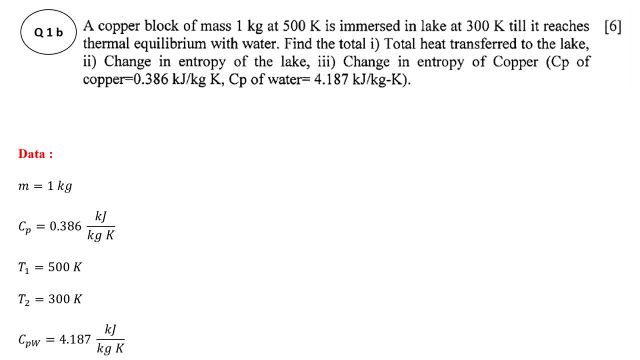 emerged is 300 kelvin and cp of water is given as 4.187 kilojoule per kg kelvin. now the first thing that we have to find out over here is the total heat transfer to the lake. so q is equal to integration of t1 to t2, mcp, dt or delta t. so mcp is constant, so it is only integration of dt. 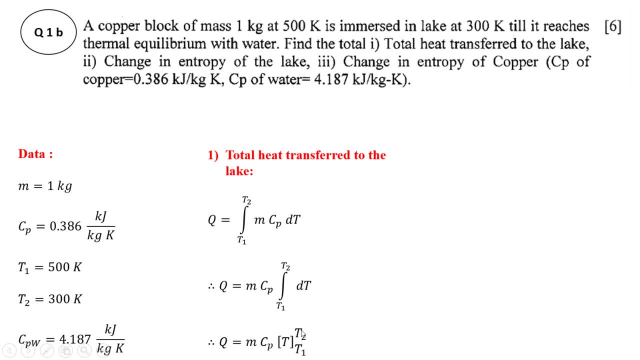 integration of dt is t and the limits are from t1 to t2. so substitute the upper limit in place of the upper limit, that is t2, minus the lower limit, that is t1. so mass is 1, cp is 0.386 and it is 300 minus 500, so q is equal to minus 77.2 kilojoule. so heat is transferred, that heat, that. 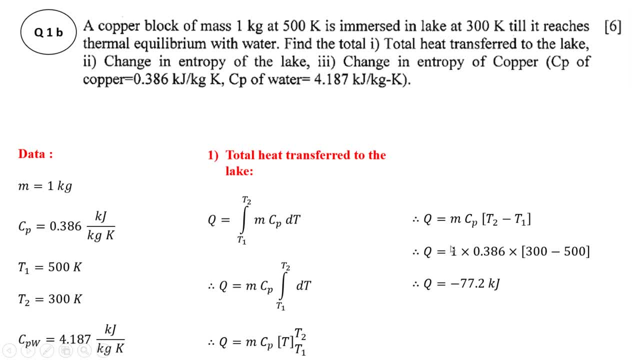 is transferred to the lake is 77.2 kilojoule and the heat is transferred from the copper block. so copper block is losing the heat and the that heat is transferred to the lake, so as the copper block, it is losing the heat. the negative sign is: 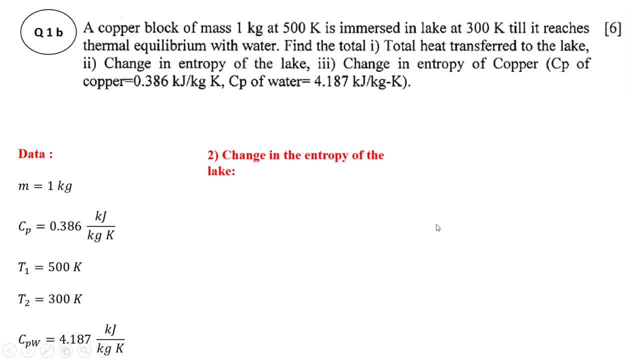 there. the second thing that we have to find out is the change in entropy of the lake. so change in entropy of the lake is equal to heat transfer to the lake divided by temperature of the lake. the lake is considered as a reservoir, so we can directly use this particular formula. 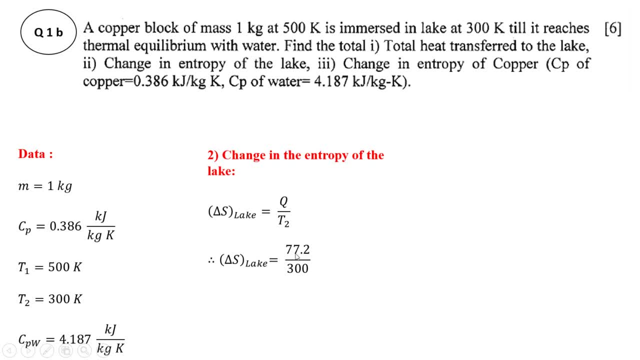 so heat transfer to the lake is positive, that is, 77.2. as the heat is received by the lake, the change in entropy will be positive and temperature- absolute temperature of the lake is 300, so it is 0.2573 kilojoule per. 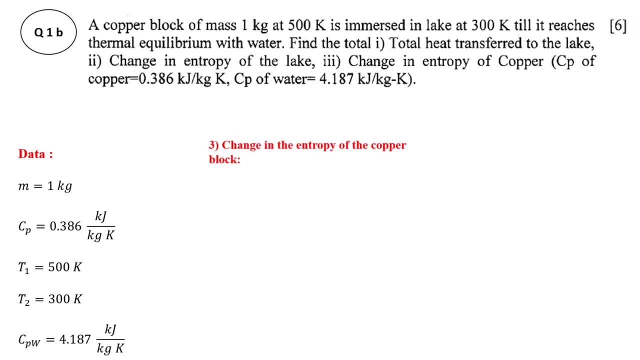 kelvin now change in entropy of the copper block. so that is given by integration of t1 to t2, dq upon t. now dq is nothing but mcp, dt, mcp is constant, so hot energy of the heat is being received by the lake. as heat is received by the lake, the change in entropy will be positive and temperature absolute.